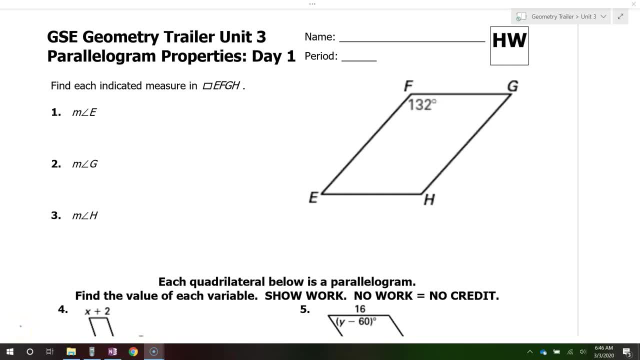 In this video I will teach you about the properties of parallelograms and we will use those properties to find unknown angles and sides and variables. So the first property I want to remind you of is that opposite angles in a parallelogram are congruent. So angles F and H are opposite angles. so this is 132. 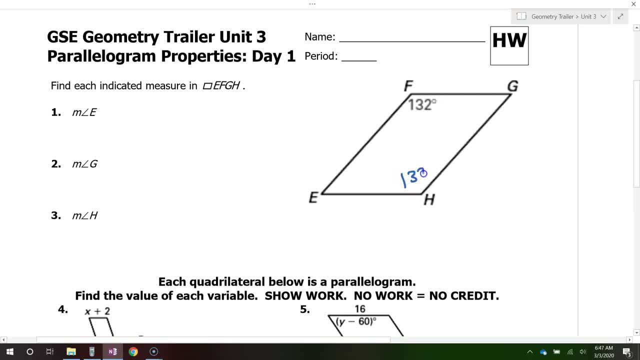 then this will be 132 degrees as well. Now, on the other hand, consecutive angles. all right, the angles that are on the same side are going to be supplementary. So this angle and this angle will be supplementary. They have to add up to 180.. 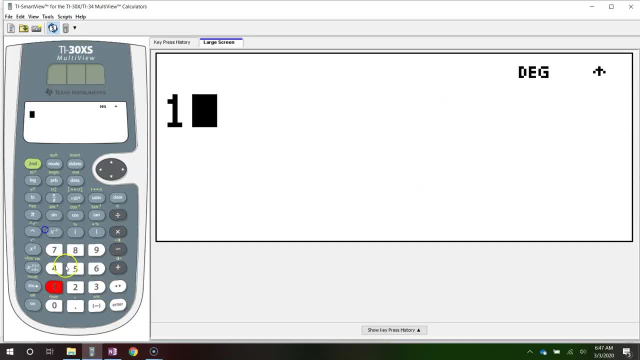 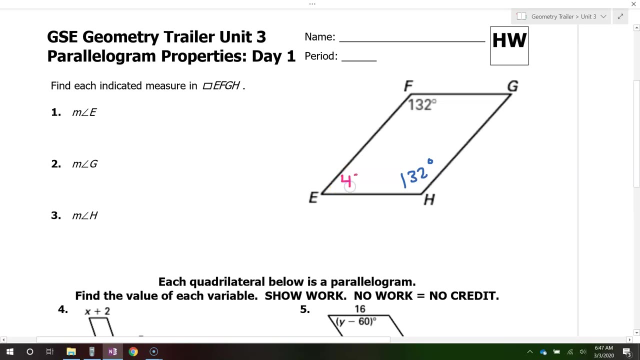 All right. so if you think to yourself, what is 180 minus 132 and, okay, 48.. So that is going to be the measure of angle E. Now, angle G is opposite angle E, and we already talked about the fact that opposite angles are congruent, So this will also be 48 degrees. It's worth mentioning that angle. 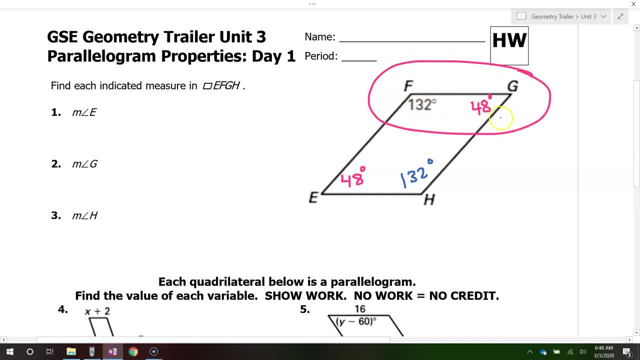 F and G are consecutive angles So they should be supplementary, which makes sense because 132 is supplementary with 48. So it works both ways. So in this way, if we have one angle given, we should be able to find all four angles easily. So the measure of angle E: 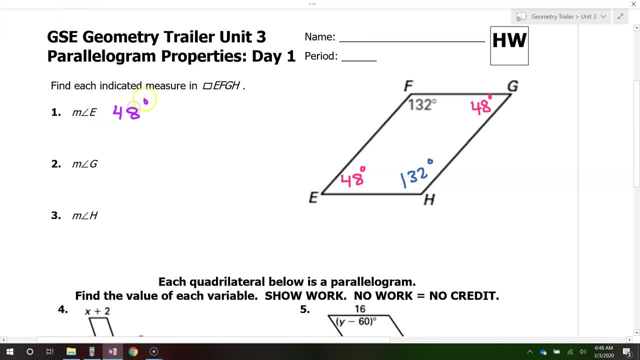 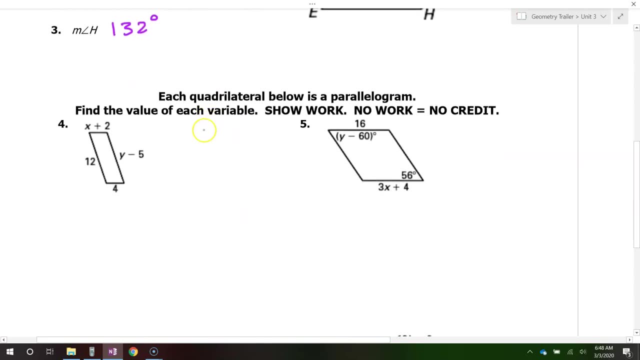 was 48 degrees, The measure of angle E was 42 degrees. The measure of angle E was 42 degrees, The measure of angle G also 48 degrees And the measure of angle H was 132 degrees. Okay, another property of a parallelogram. 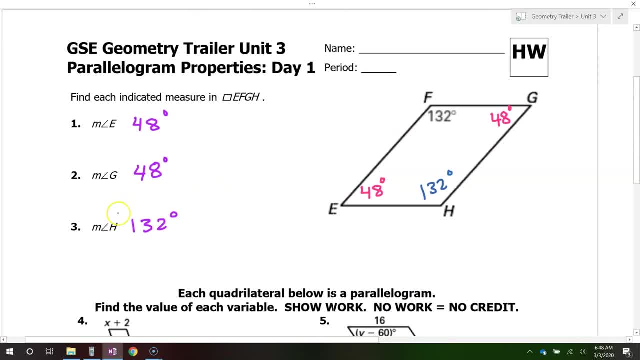 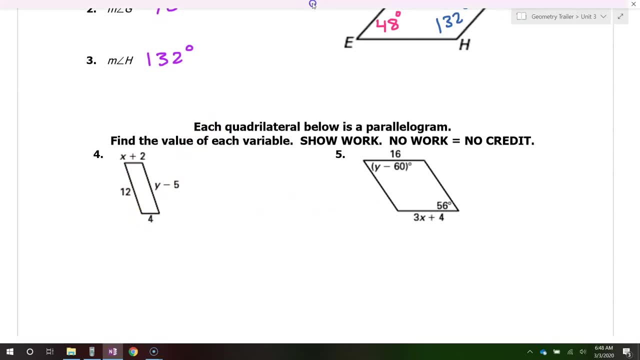 is that opposite sides are congruent. So opposite angles are congruent, but opposite sides are also congruent. So for that reason, X plus two should equal four, because those are opposite sides. So I can use that to make a little equation. 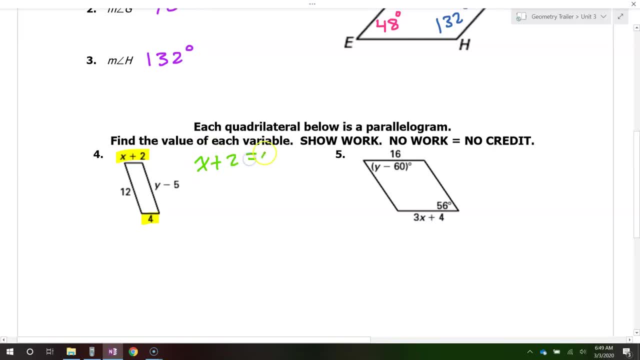 So I could say X plus two should equal four. Of course, if we subtract two from both sides, I get X equals two. If I wanna find the Y value, well, these are opposite sides, So those should be equal to each other. 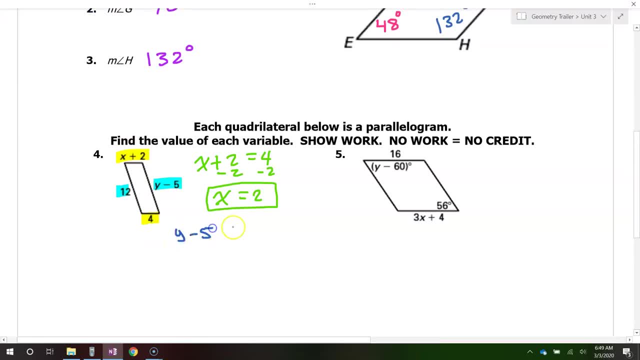 So I can say Y minus five should equal 12. Then if I add five to both sides, I get Y equals 17. So we found that variable Okay. so this next problem has a combination of opposite angles and opposite sides. In both cases these should be equal to each other. 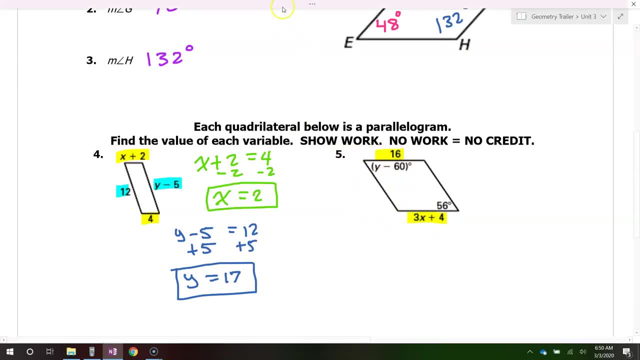 Opposite sides are equal. So from that I get the equation: three X plus four will equal 16.. Well, let's solve it out. Subtract four from both sides, That gives me three X is equal to 12.. And then divide both sides by three. 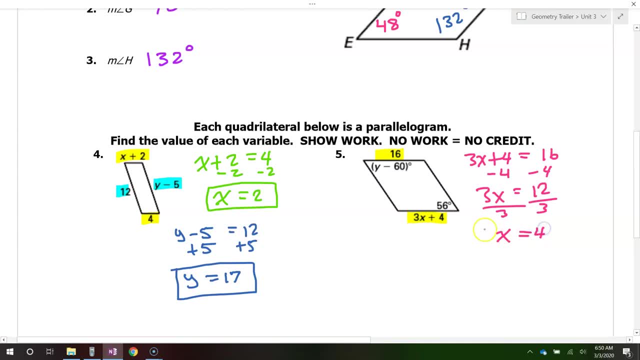 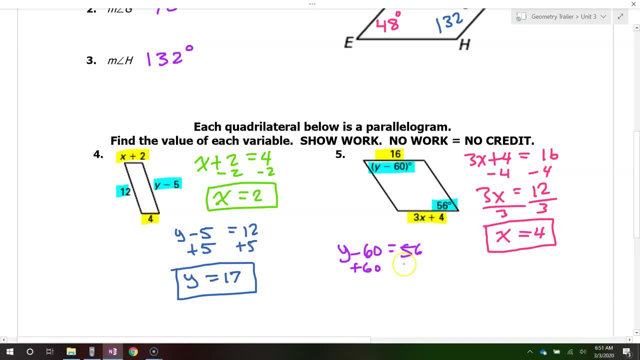 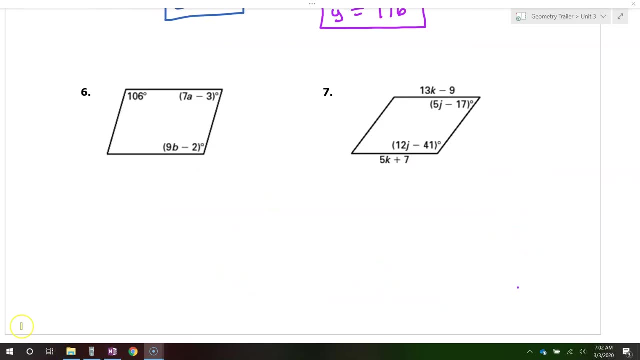 So that's gonna tell me that Y minus 60 is equal to 15.. So if I add 60 to both sides, Okay, that's gonna give me 116.. For number six, we're gonna use the fact that opposite angles are congruent first. 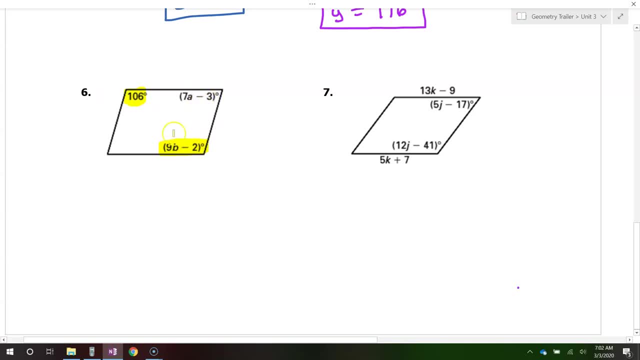 Instead we have consecutive angles angles. I guess we could have done either one. but 9b minus 2 should definitely equal 106, and then we will add 2 to both sides, so that will give us 9b is equal to 108. so when we divide both sides by 9, we're going to get b is equal to 12. all right, now we 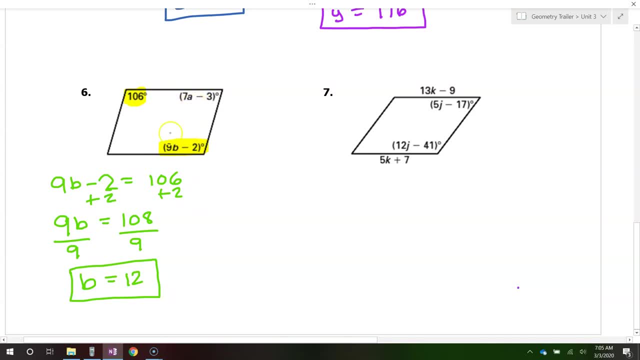 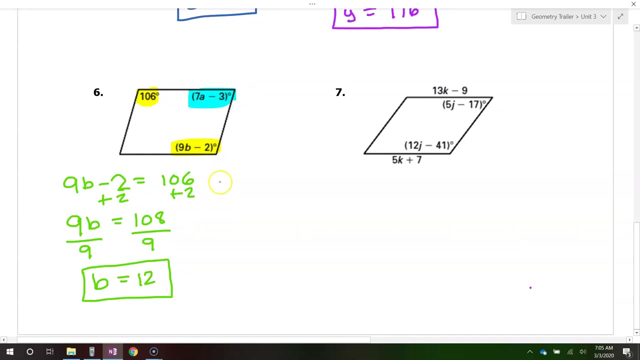 still need to find the a value. so let's use the fact that consecutive angles are supplementary. all right, so that means that this yellow and blue, they should add up to 180. let's see. all right, so that's going to look like this. we will say 7 a minus 3 plus 106. 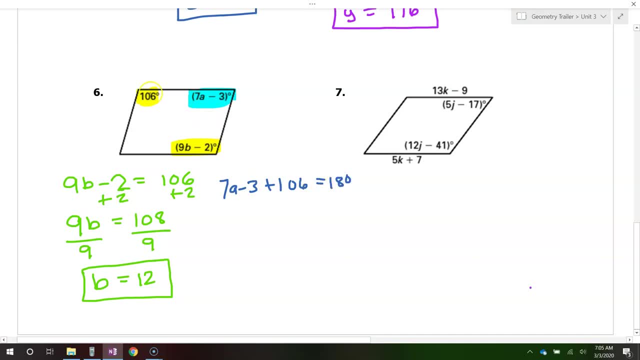 is equal to 180. right, these two angles are supplementary. well, let's combine these like terms first. they are on the same side, so we simply combine them. so we have 7 a plus 103 is equal to 180. we can then subtract 103 from both sides, so that will give us 7 a. 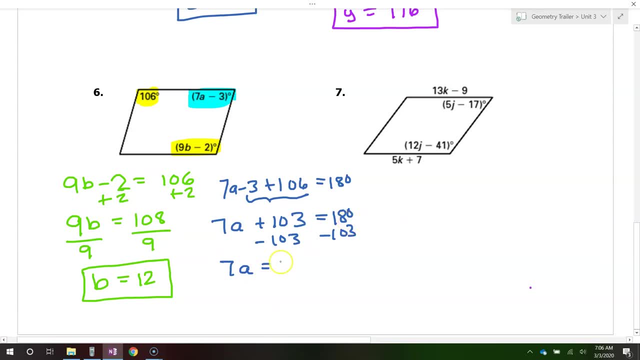 plus 106 is equal to 7d7, of course. then when we divide both sides by 7, we get a is equal to 11. all right, one more problem. first, let's use the opposite sides, or the fact that opposite sides of a parallelogram are congruent, so these will be equal to each other. so we can go ahead and say: 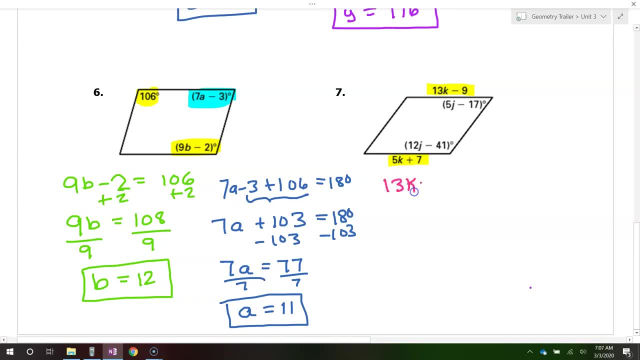 that 13k minus 9 will equal 5k plus 7. so we have the variable on both sides of the equation. so we need to subtract 5k from both sides to get those k's together. okay, so that is going to give us: 8k minus 9 is equal to 7. next we would add 9 to both sides so that 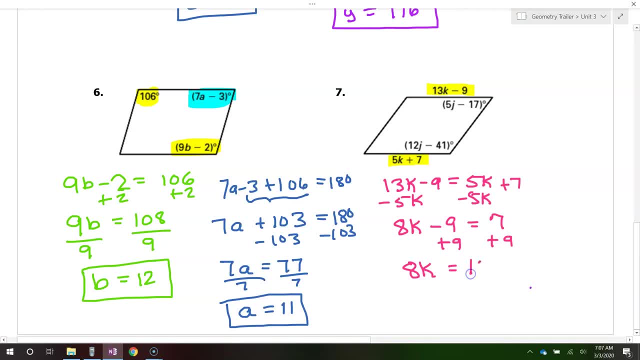 will give us: 8k is equal to 16. so finally, when we divide both sides by 8, we're going to get k is equal to 2. all right, and now let's use the fact that consecutive angles are supplementary. so please be careful, these two angles inside of here they are not congruent. 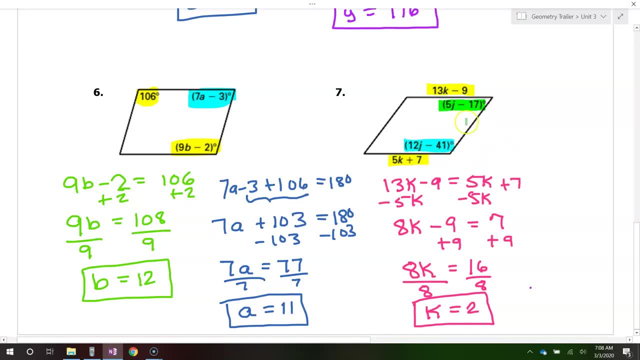 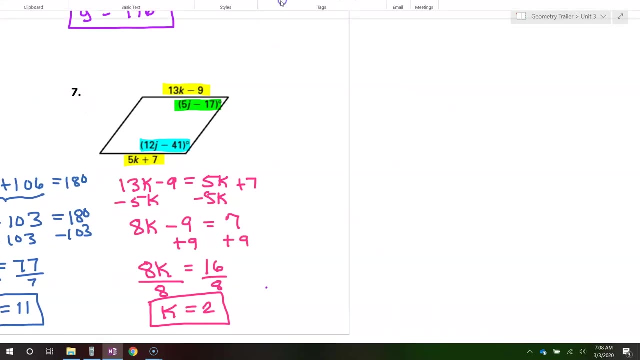 they're, because they're not opposite angles. they are on the same side of the parallelogram. the green one is acute and the blue one is obtuse, so they are not congruent. they are supplementary, so they need to add up to 180. so what we can say is that 12j minus 41 plus 5j minus 17 should. 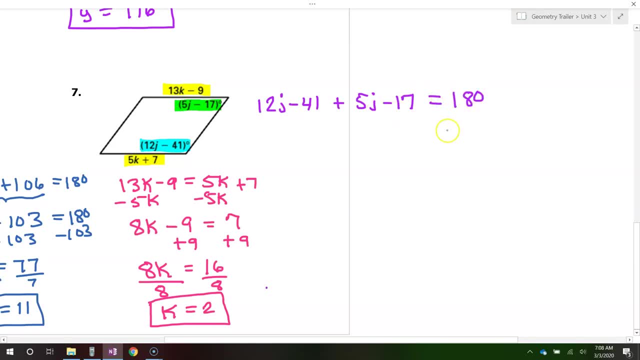 equal 180. all right, they are supplementary, they add up to 180. now all of these terms are on the same side of the equation, so we're just going to combine like terms. so, looking at the 12j and the 5j: all right, those are like terms, so let's just put those together. so that's going to be 17j all. right. and then, of course, we're going to add up to 180, so that's going to be 17j, all right. and then, of course, we're going to add up to 180, so that's going to be 17j, all right. and then 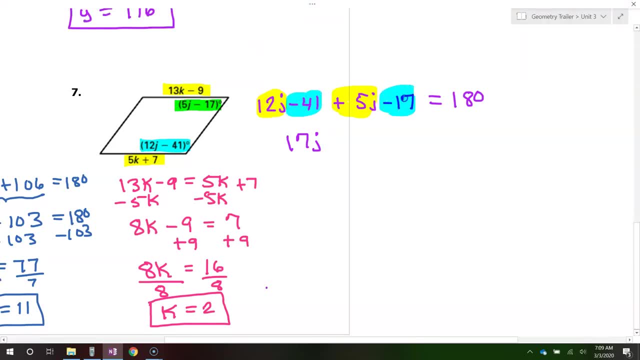 also combine the negative 41 and the negative 17.. okay, so that's going to give us negative 58 and that will equal 180. then, of course, if we add 58 to both sides, we wind up with 17j is equal to 238. so finally, we will divide both sides by 17 and that will leave us with j equals, whatever that is. 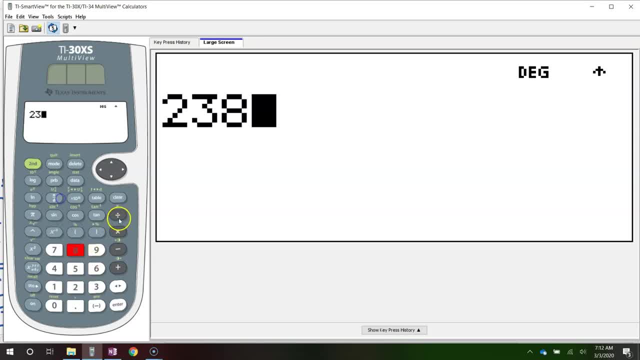 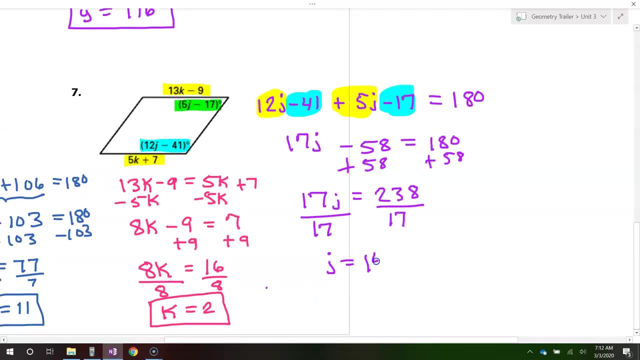 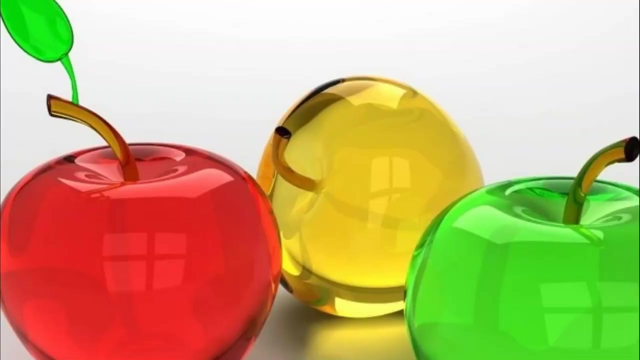 all right, and that is 14.. so that is how you use the property of the properties of parallelograms to find unknown values. all right, all right, so the social gap over here. this is an Painter's way and it will be n over n. So you keep going out by sword. oh, it should beこちらが and get this and get this and a plus, All right. And then I just see the square: There you go.